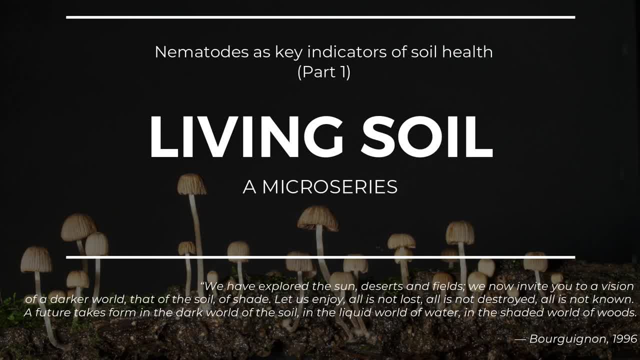 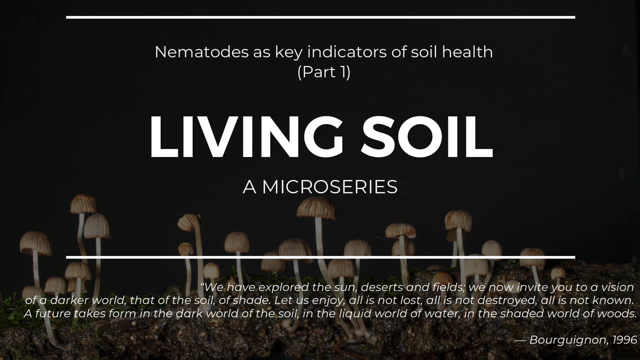 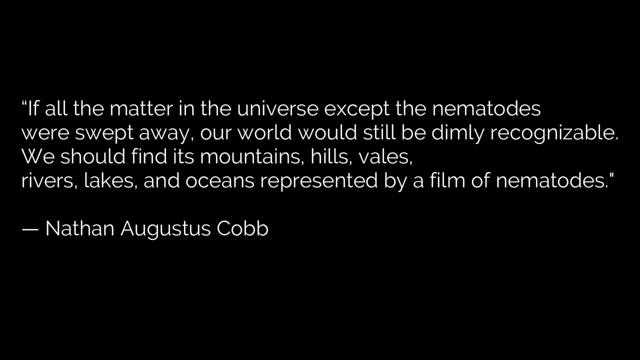 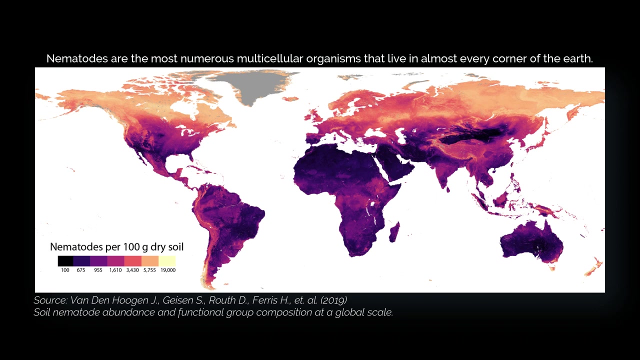 Nematodes. Nematodes are the most numerous multicellular organisms that live in almost every corner of the earth. They are incredibly diverse. They are found in soil, water and even inside other animals. Most fertile agricultural soils have at least 5 million nematodes per square meter. 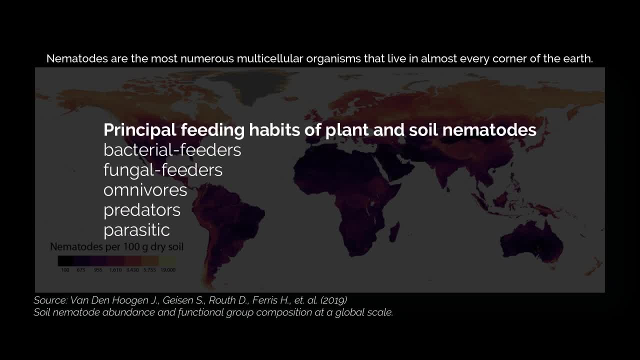 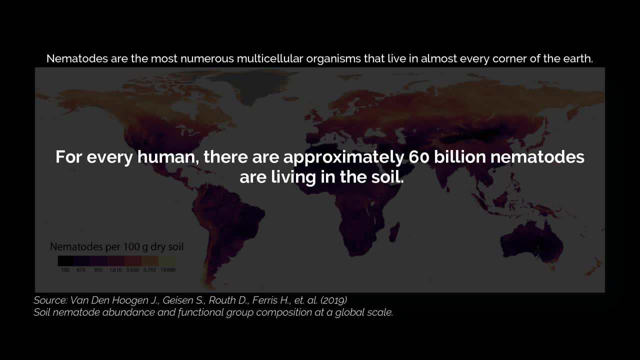 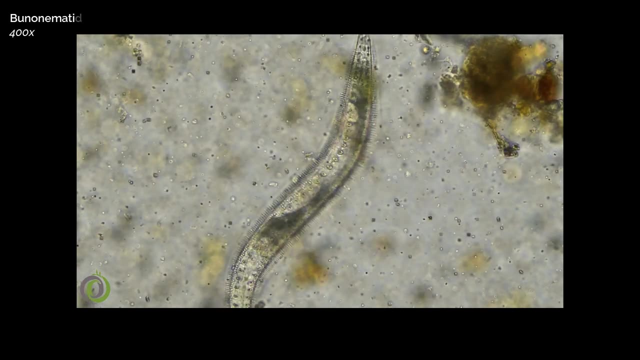 They feed mainly on bacteria and fungi, but plant, parasitic, omnivorous and predatory species also occur. For each human, approximately 60 billion nematodes are living in the soil. The soil environment is a major source of nematode diversity, with 42% of the species described. 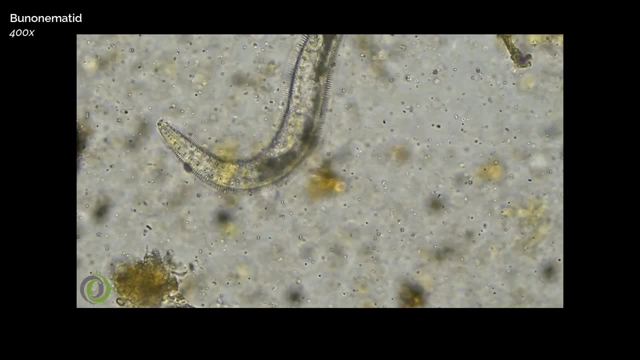 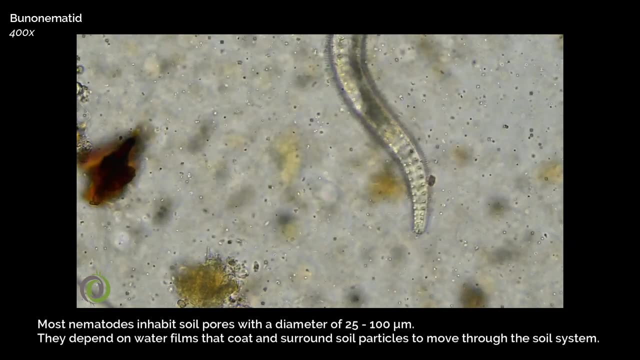 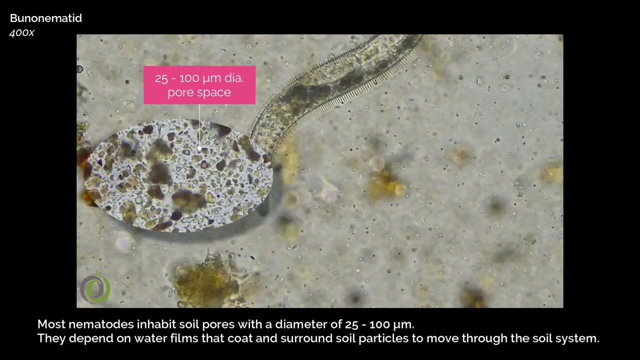 being terrestrial, They cannot reshape soil, so they must use existing pore spaces, water cavities or channels for locomotion. Most nematodes inhabit soil pores with a diameter of 25 to 100 micrometers. They depend on water films that coat and surround soil particles to move through. 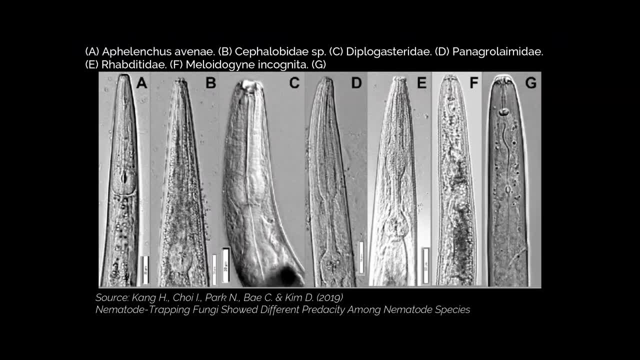 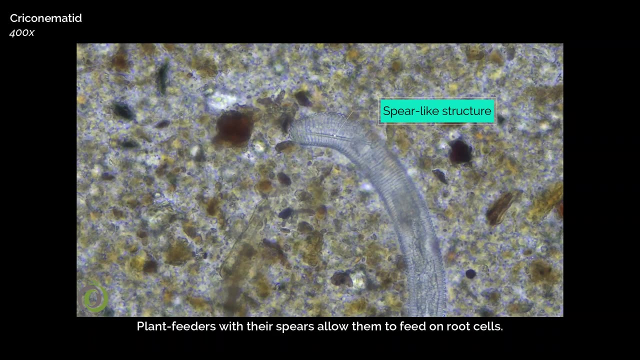 the soil system. Learning about the different groups of nematodes and their eating habits is fascinating. You can identify what they eat by examining the shape of their head, For instance. nematodes that consume plants have a spear-like structure that allows them to feed on root cells. 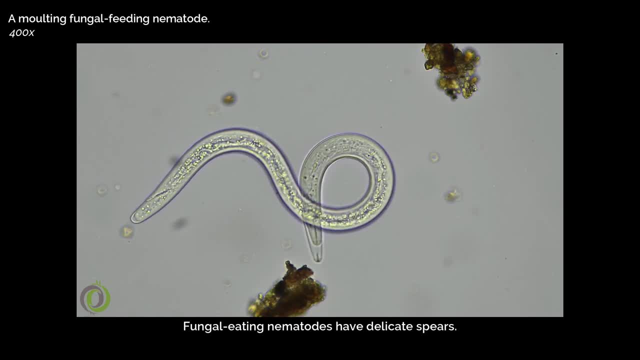 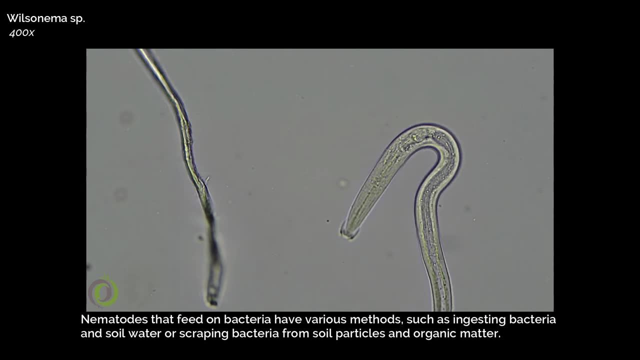 Meanwhile, fungal-eating nematodes have a more diverse diet. They have a more delicate spear that enables them to penetrate cell walls. Nematodes that feed on bacteria have various methods, such as ingesting bacteria in soil, water or scraping bacteria from soil particles and organic matter. 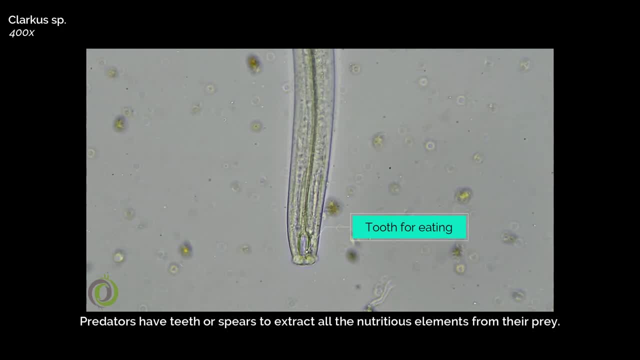 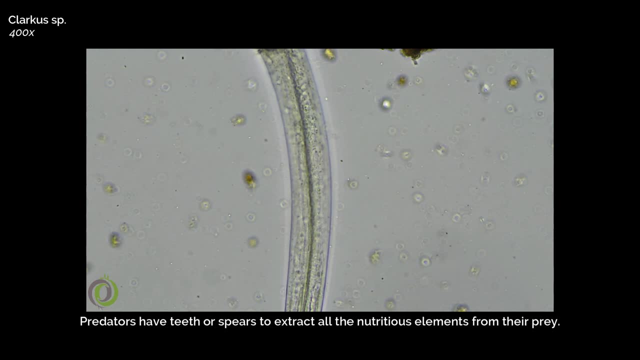 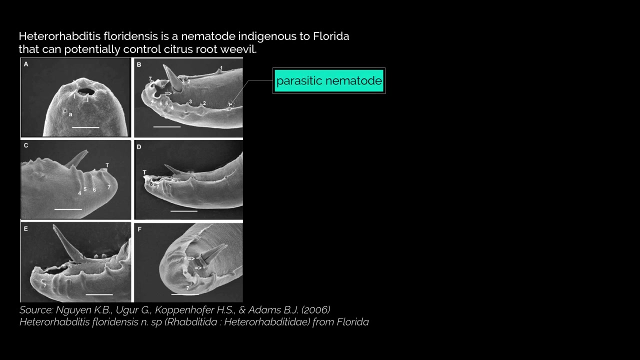 Predatory nematodes possess teeth to feed on other nematodes and small animals, while omnivorous and some other predators have spears to extract all the nutritious elements from their prey. Parasitic nematodes are especially skilled at infecting their insect hosts. They are essential.